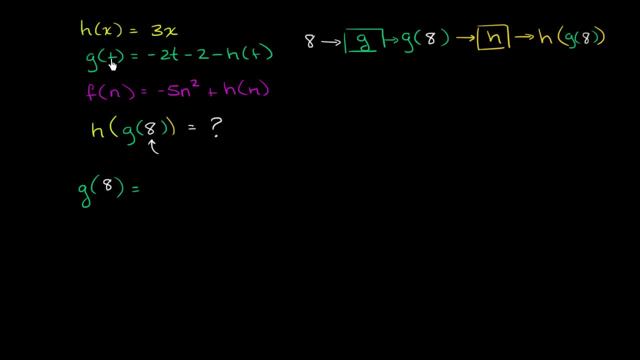 g of t. we have our definition here, So our input now, instead of a t, 8 is going to be our t, So our input is 8.. So every place where we see a t in this function definition, we replace it with an 8.. 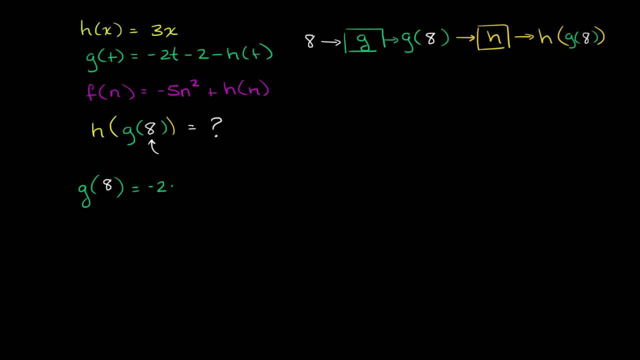 So it's going to be negative 2 times 8 minus 2 minus, and this might be a little daunting, but let's just replace this t with an 8 and then see if we can make sense of it: h minus 2 minus h of 8.. 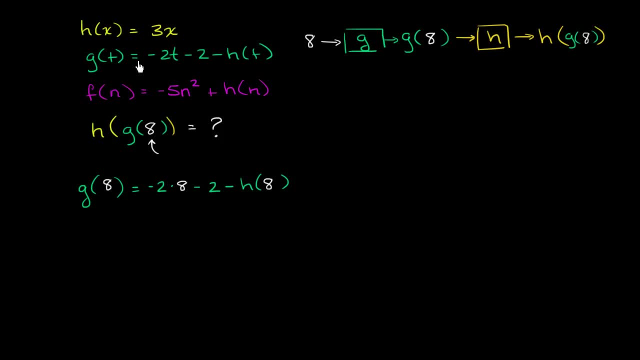 Notice to evaluate g of 8, all we did is, everywhere we saw a t, we replaced it with the input 8.. Now let's see if we can calculate this. This is going to be equal to negative 2 times 8. 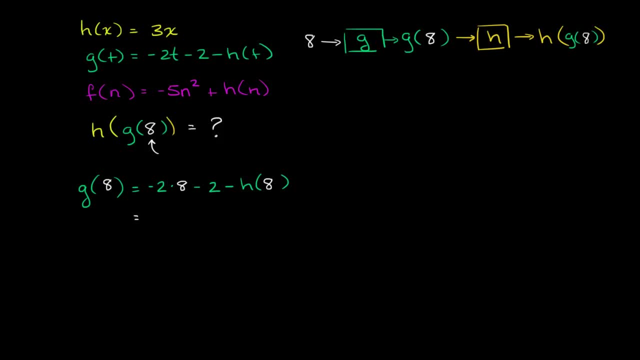 is negative. 16 minus 2 is negative 18.. Let me do that same. So this is going to be: t equals negative 18 minus what is h of 8 going to be equal to. So let's do that over here. 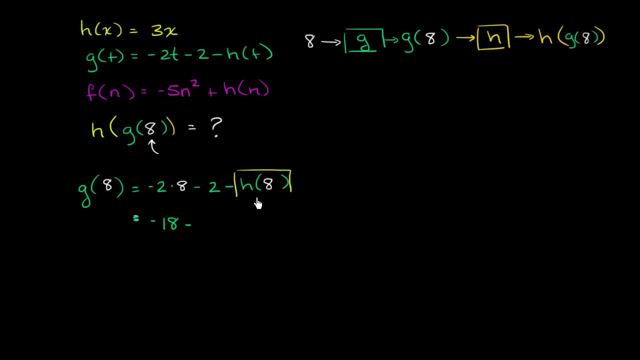 So h of 8, this thing, h of 8.. Now we go to the definition of h. Don't worry about later we're going to input all this business into h again. Just let's worry about it one step at a time. 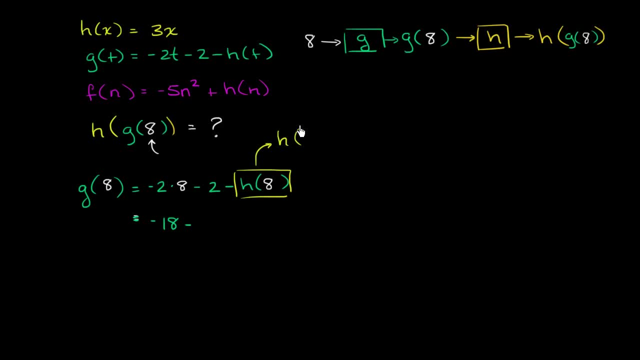 We need to calculate h of 8.. So h of 8 is just going to be. well, every time we see an x, we replace it with an 8.. It's going to be 3 times 8, which is equal to 24.. 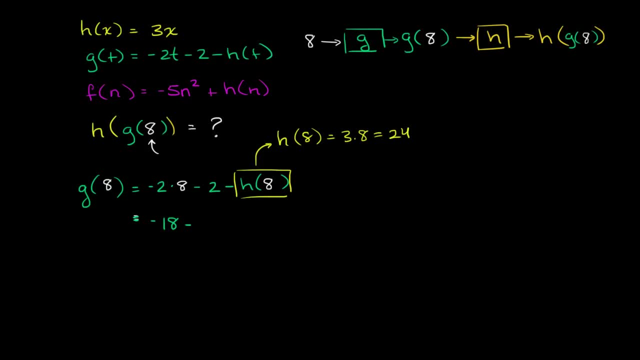 So this value right over here is 24.. We are subtracting it So we have minus 24.. Negative 18 minus 24 is what That's negative 42. So all of this business is going to be equal to. did I do that right? 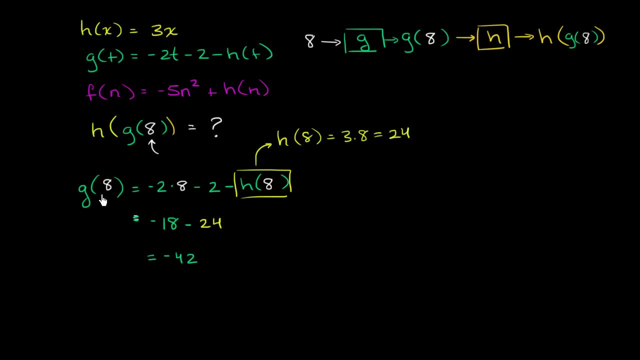 Yeah, negative 42. So we figured out what g of 8 is. It is negative 42. So this right over here is negative 42. And now we can input negative 42 into h. So h of- let me do it right over here- h of negative 42..